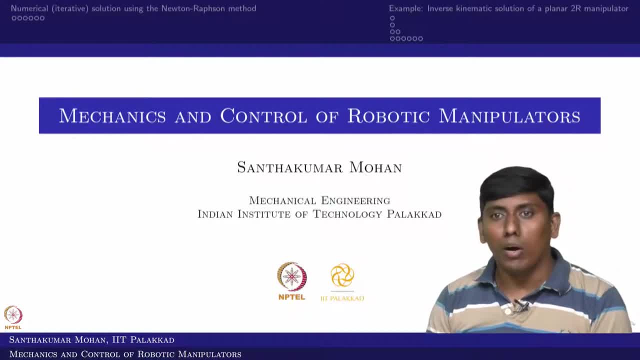 representation In the same lecture. I was actually like, given a small idea, so, with the help of solve command, how to find the inverse kinematic solution if you have forward kinematic solutions are available In the sense if you have mu vector. so how we can actually like. 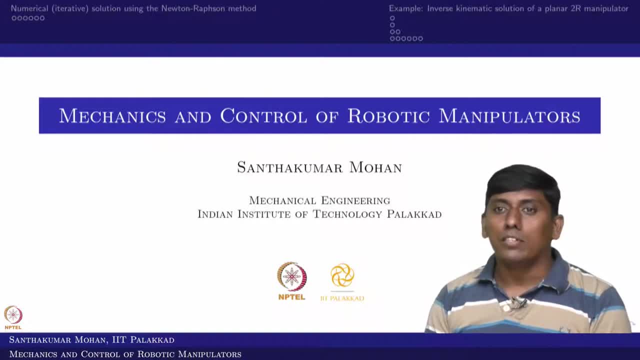 find the inverse kinematic solution using solve, But the solve is not the right option all the time, so we use- actually like a numerical method which is faster. so that would be beneficial when you do for online programming and other things. For example, you have a robot in real time, so obviously the numerical method would be. 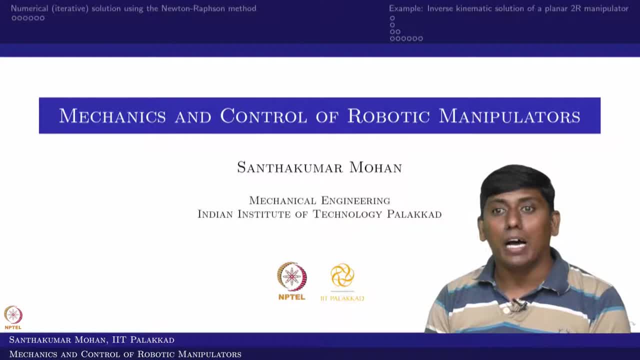 little more beneficial than the closed form solution in the, you can say, computational perspective. So in that sense, this particular lecture is going to talk about how to use Newton Raphson method for finding inverse, inverse kinematic solution of a serial manipulator. So here again, the same example which we have taken in the original lecture. The same example. 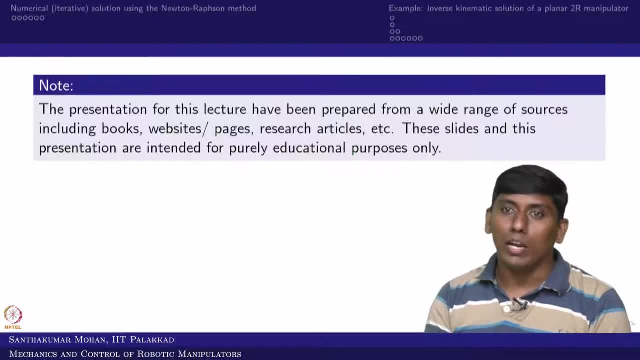 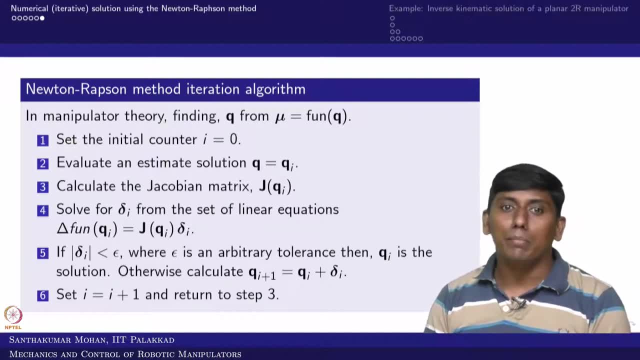 two are: planner, serial manipulator we have taken trying to derive the code with the help of the algorithm which we have come across. So only change what we made is, instead of this, delta i, we are going to take the relative tolerance or the arbitrary tolerance we are going to take, instead of delta i, we are going 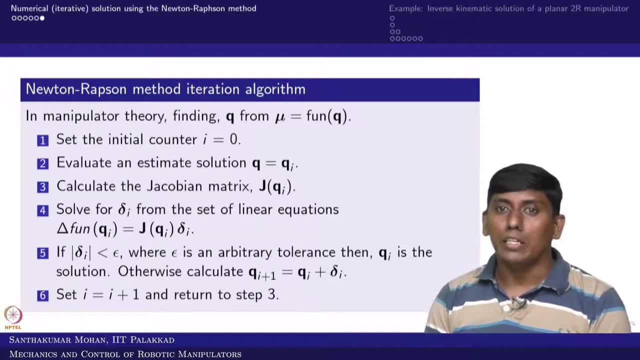 to take delta mu. okay, that is the only thing, because delta i would not be available to us. So we would be seeing that. what other error we can restrict? we can restrict the delta mu. that is the only restriction we are making. it other than this: you can say: algorithm which: 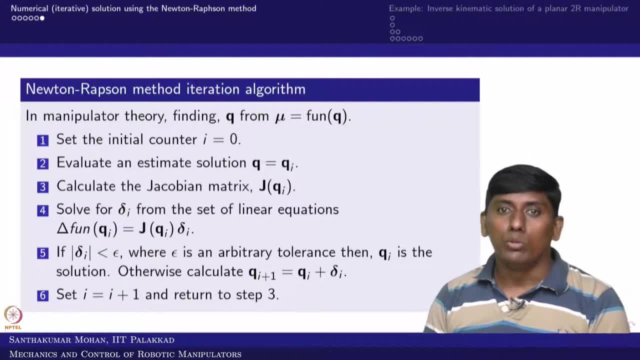 we have written, In addition to that, what we supposed to know. we should have the j of qi and q, initial guess, and mu mu is actually like function of q. these all need to be known. So in that sense, what we can actually see if we write the MATLAB code for this 2R serial. 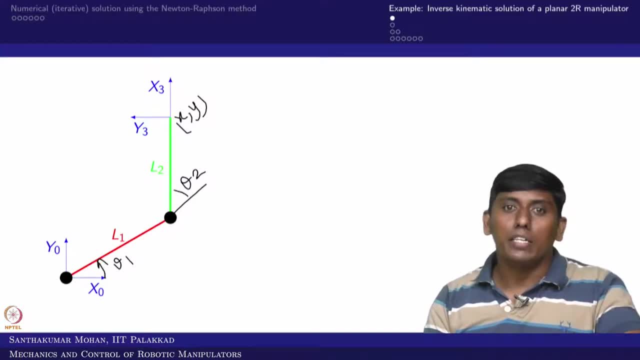 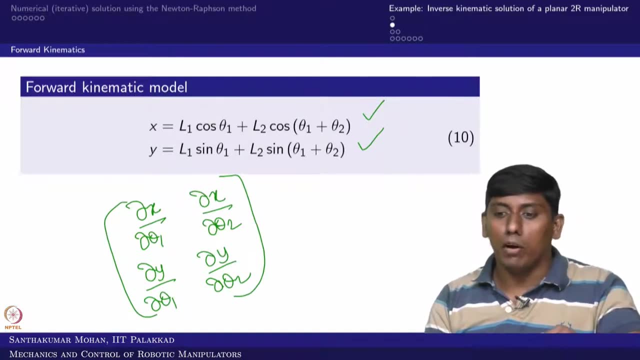 manipulator. if the x and y are known, can we find theta 1 and theta 2.. So for that you know this equation. So where x and y would be given, as in the form of function of q, here theta 1 and theta 2.. 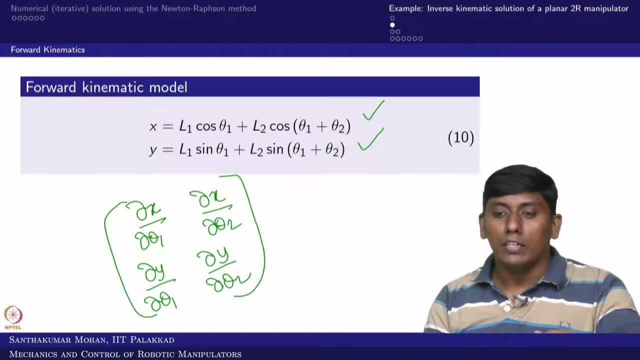 So if this equation is known, then we can find the Jacobian matrix in the order of, or you can say, in the way of partial derivative which I have written in the board. So now, if we see that this partial derivatives are available, can we actually like cross check? 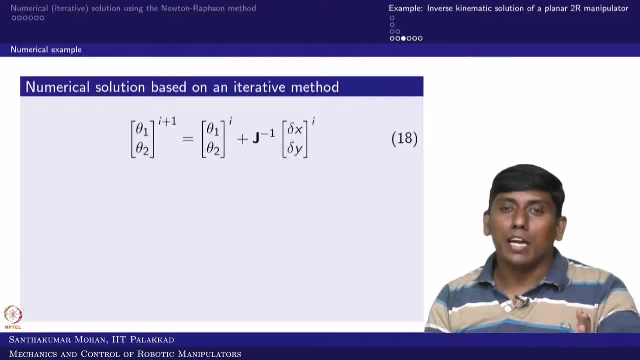 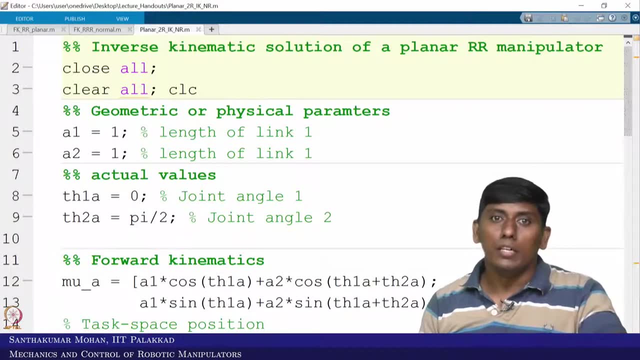 the closed form solution. whatever is giving the result, the same result can be obtained with the iterative method. So for that we have actually like taken the code, which is we have already written. ok, So you can see that the initial command all are same. So this is inverse kinematic solution of a planar RR manipulator with the help of iterative. 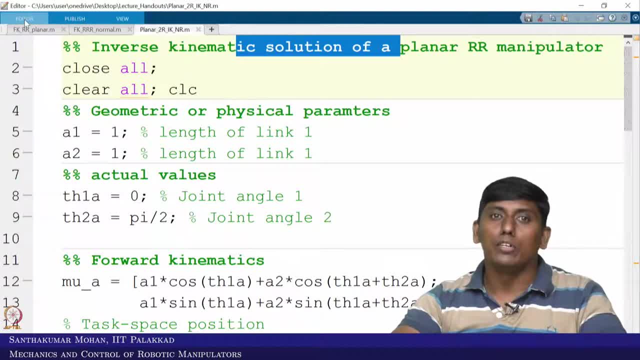 thing. So only issue is actually like I make the editor window closed. ok, So this window is actually like I closed just for my benefit so that the display would be very much visible for you, but whenever you run, so you can go to editor and you can actually. 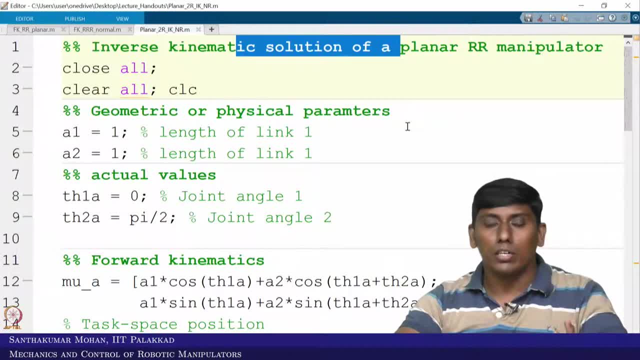 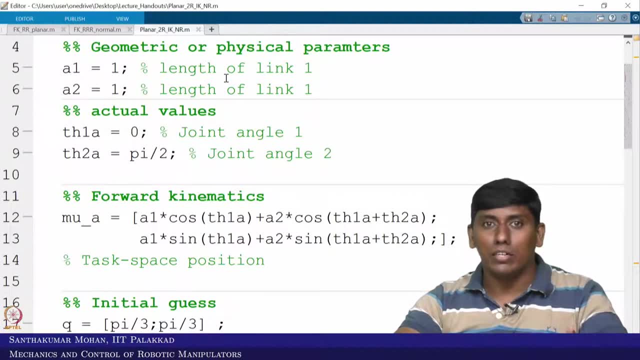 like run, Run and advance, but I am going to use a shortcut, what called F5. ok, So now this is actually like the standard. So now we are actually like seen in the lecture, So where L1 and L2 are actually like one unit each. 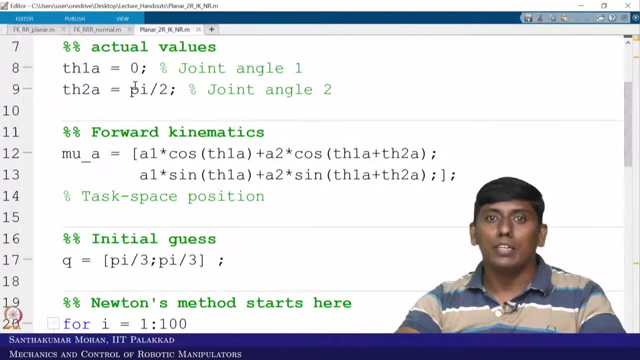 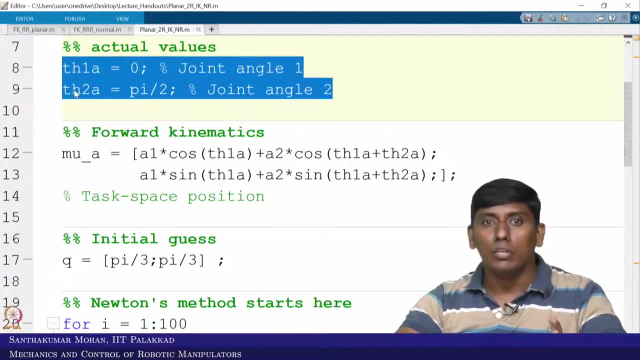 So the same thing, we are actually like taking it. So again, I am actually like seeing one given point. So in the sense, this is in actual we do not know, but for finding the mu value, I am actually like assuming that this is the actual angle in the sense. 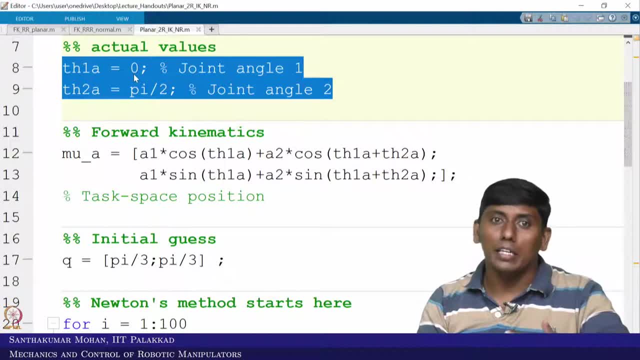 So I am actually like making Theta 1 is 0 and theta 2 is 90. What would be the mu that is, I am assuming, as a given mu value? So in the sense, this is not really there for us. So for us, actually, this is obtainable in the sense. 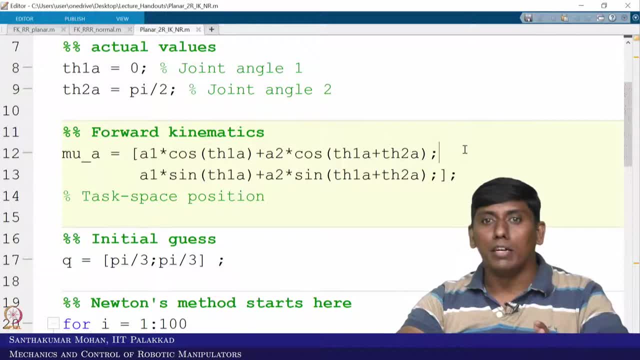 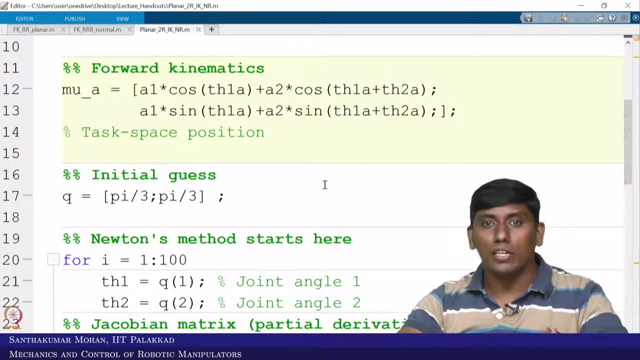 So, instead of this relation, the mu A would be straight away given. So in this case it is 1, 1, ok, So then what we are trying to do? as per the algorithm, we have to start with the guess. So I am taking a guess as so pi by 3 each. 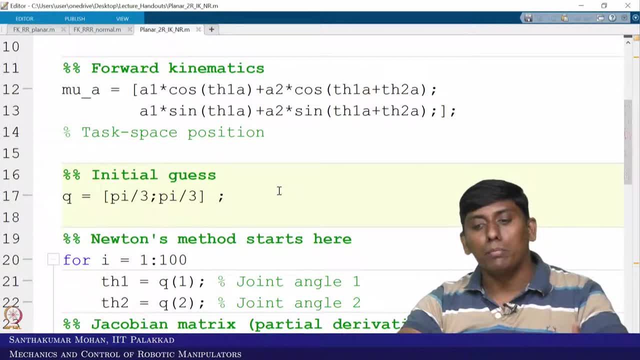 So after that I am putting, the iterative count is actually like it can go up to 100 count, But it may not required. I am saying that the maximum count can go to 100. ok, So for your benefit, I am restricting to 10. ok. 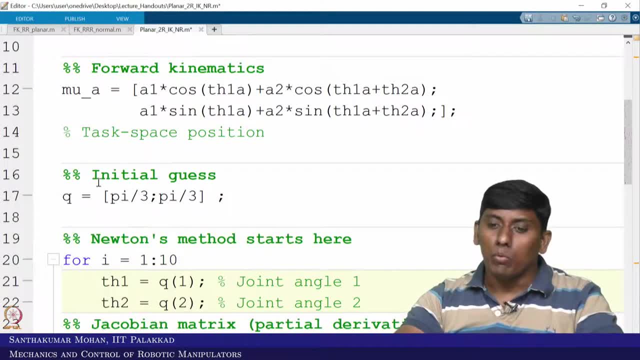 It is nothing going to change. So then what I am saying? that whatever I am actually like, taking a initial guess that would be equal to theta 1 of you can say the first value would be theta 1, second value would be theta 2.. 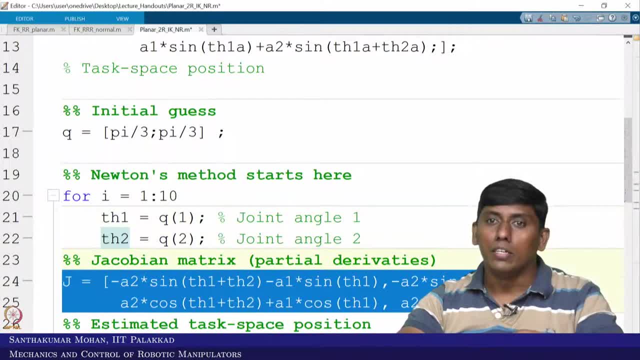 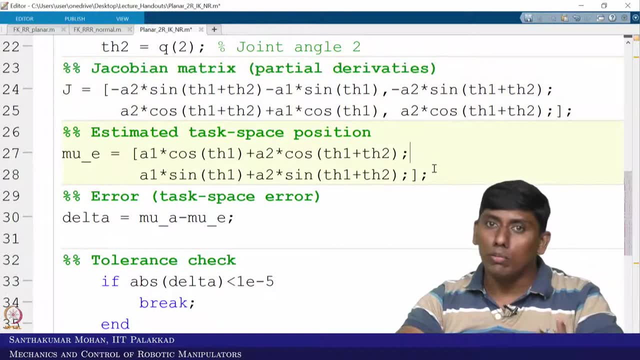 So then I am actually like derived already with the partial derivative as what you call The Jacobian Jacobian matrix. So this Jacobian matrix I have derived. So after that I am actually like know the forward kinematic relation, So which will give the mu estimated ok, 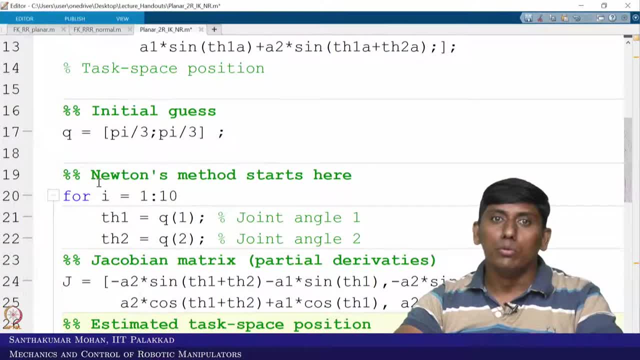 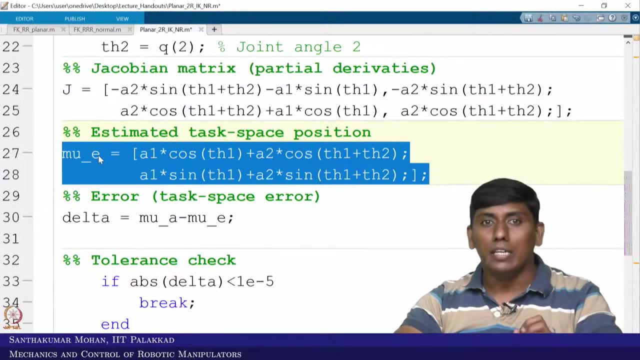 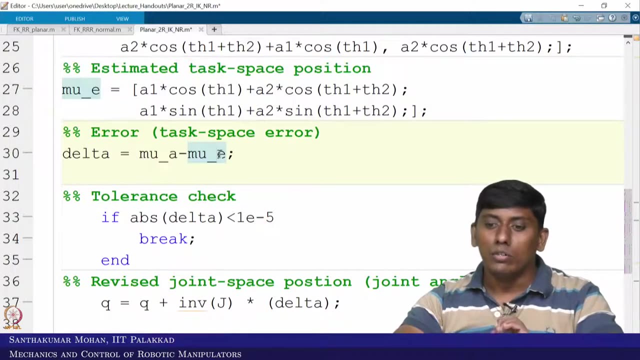 So the mu underscored E is actually like mu estimated. So the mu actual mu underscored A. So now the mu underscored A – mu underscored E is actually like your delta mu. So that is what I have written as delta. So the delta is actually like actual minus estimated. 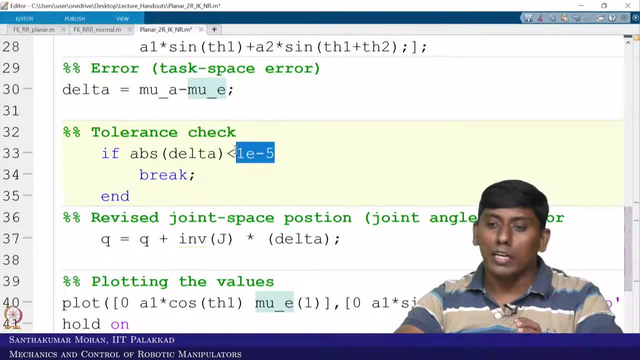 So now I am putting a tolerance check, So, which is actually like 10 power minus 5.. So the absolute value is actually like less than or you can see, or equal to 10 power 5.. So 10 power minus 5.. 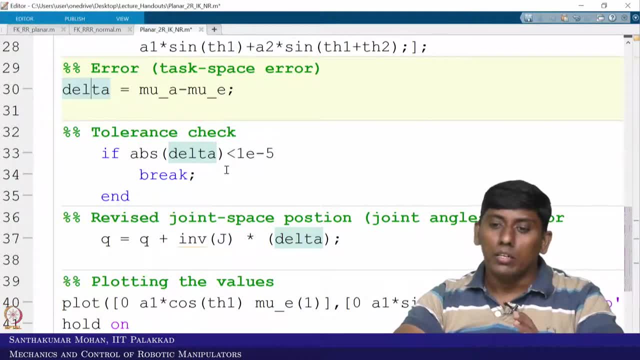 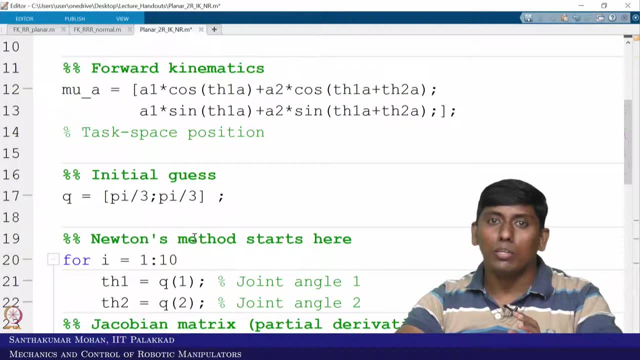 So then you break the algorithm. ok, So break the code In the sense. stop and give the final result, otherwise you still keep on going Again. we have restricted. the total iterative count is 10. right In the sense. if this is actually like not matching, this will run up to 10 and says that. 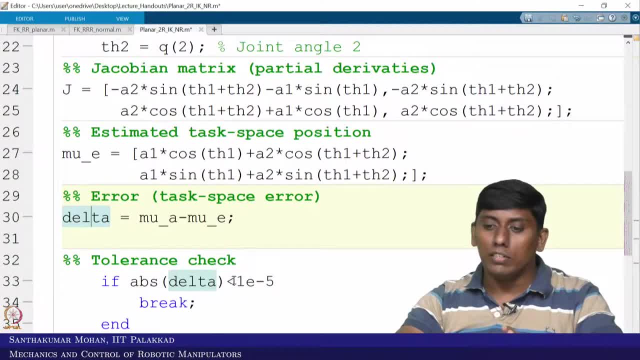 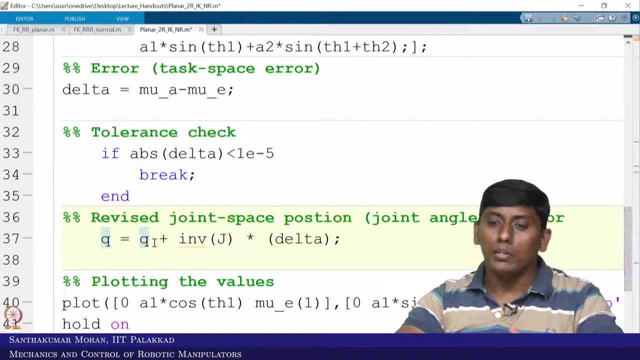 this is the final result. It is not matching. Ok, If this is the case, it will give the final match. So now what we are doing it. So the q i plus 1 is actually like q of i plus inverse of j, multiplied with the delta. 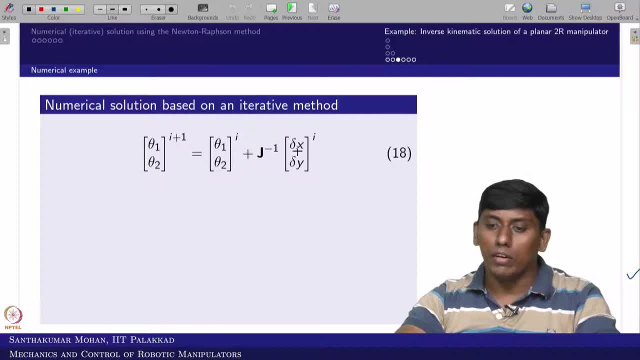 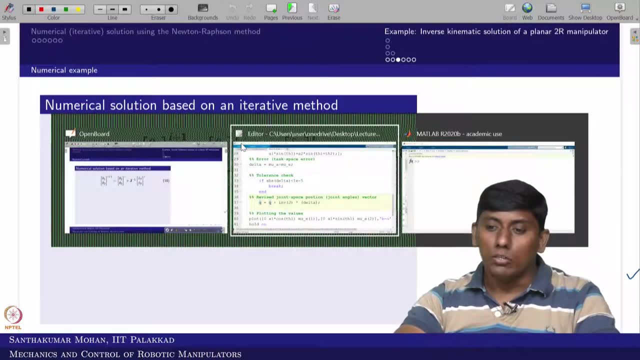 ok, So you can actually like recheck. this is the code. we have actually like written it right. So this is the same thing. So, instead of i plus 1 and i, I have denoted as q itself. So maybe it may be little confusing for you, but I do not want to keep. the count is actually. 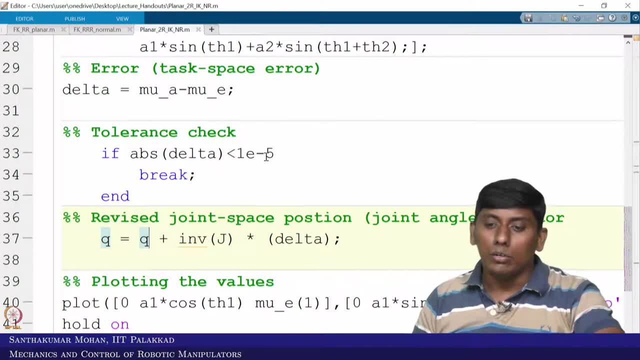 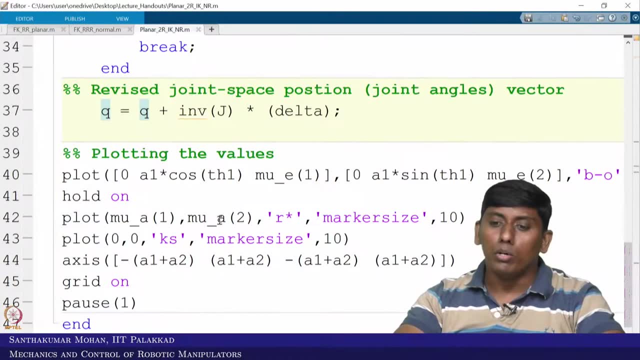 like iterative In the sense x would be giving a multiple. you can say array, So that I do not want. So q keep on actually like getting change. So once this is known, I want to actually like plot. So for that I am just drawing a 2 r serial manipulator. 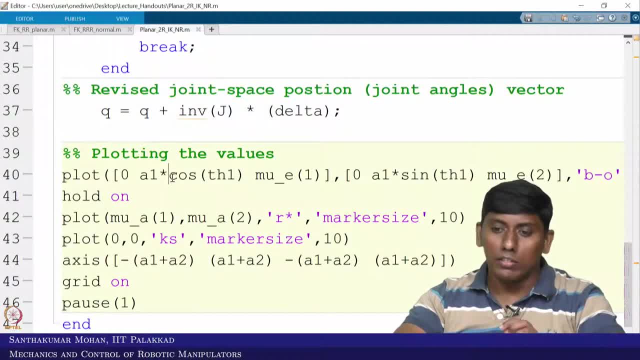 So, which is actually like I have, take origin, then the first joint position, in the sense that is the origin. second joint position and the end effector: ok, this is the x 0, x 1 and x 2. ok, In your case it is supposed to be: x 0 and x 1 is same, x 2 and x 3: ok, 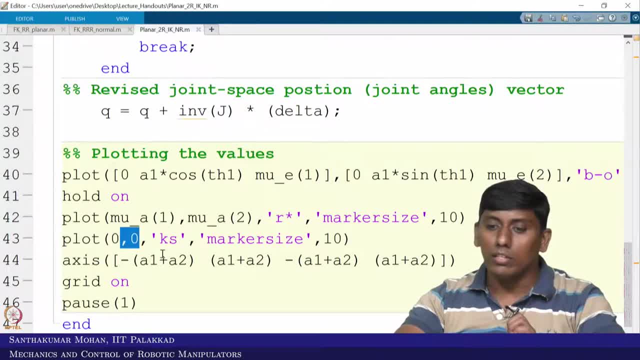 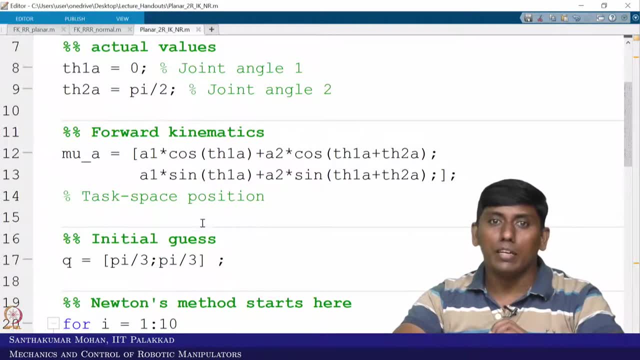 So then I am actually showing this is the given value and this is origin, how my actually like count is actually like keep changing that. it would be showing it. So right now, what we have taken, we have taken a random guess which is pi by 3 each. ok, 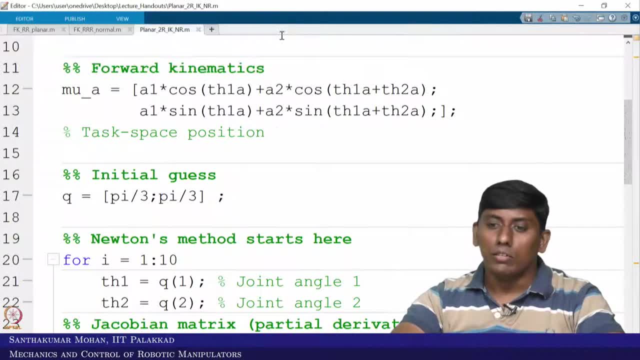 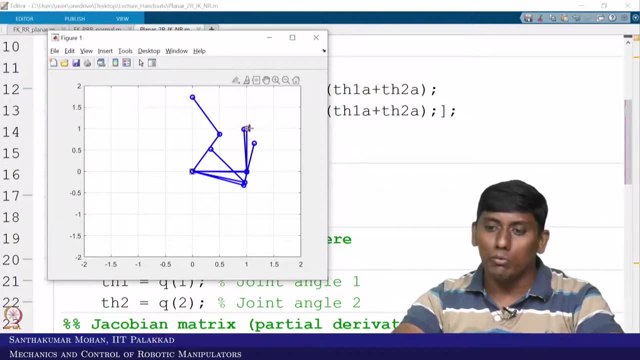 So now, if I actually like run through this, ok, So I will see that the output, you can see that. So this is the initial guess. So actually I keep going. this is the final outcome. you can see it, it is coming right. So it actually like gone something and it reach. 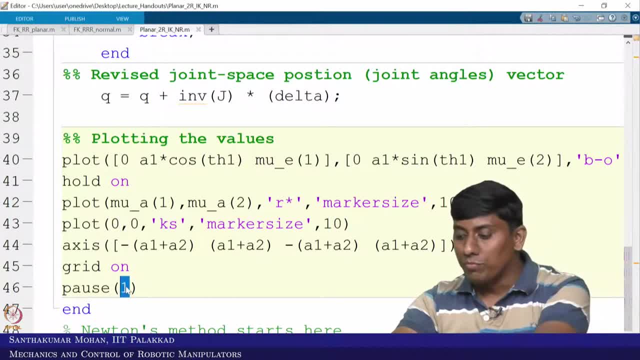 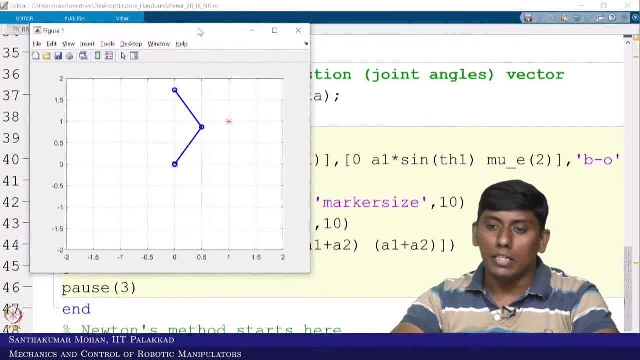 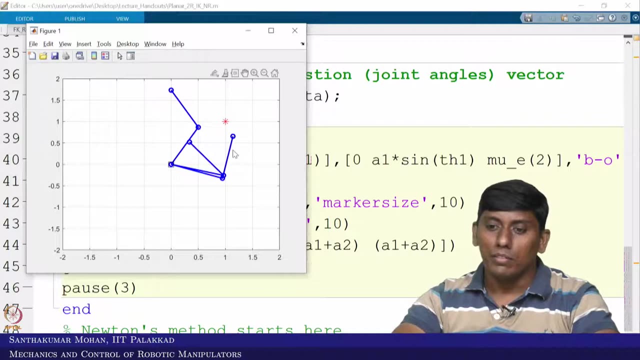 So I will actually like keep the time little higher So that I can actually like show it. ok, So now I put 3 second for a delay, So you can see. So this is the first one. This is the second iteration. ok, this is the third iteration and the fourth iteration it. 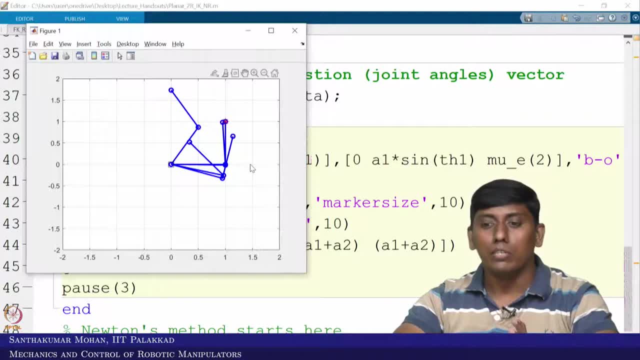 is closer. And fifth iteration: Yes, Almost reach the relative tolerance which you have given. So now, this is 1 comma 1, and you have actually, like, made it right. So now, if I take the non, you can say, for example, different initial guess. 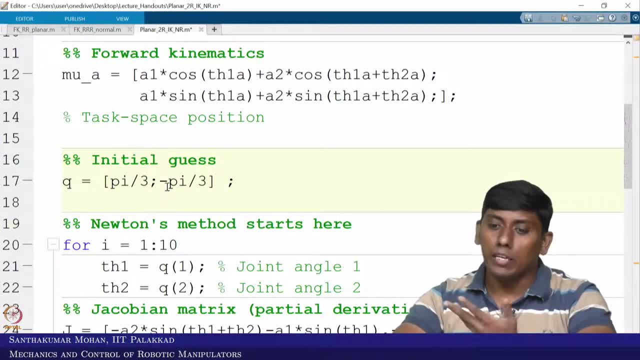 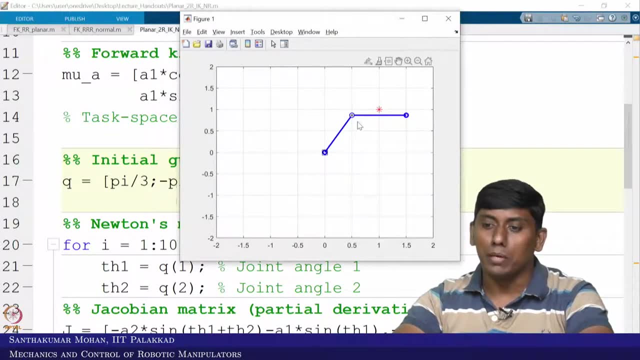 I am taking pi by 3 minus pi by 3.. So we expect the final solution to be converge, but which solution we do not know. You can see now. it started minus pi by 3 in the second joint. this is the second iteration and third iteration itself. it is converge, right. 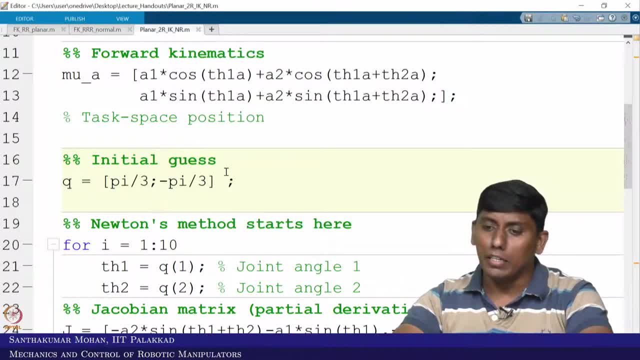 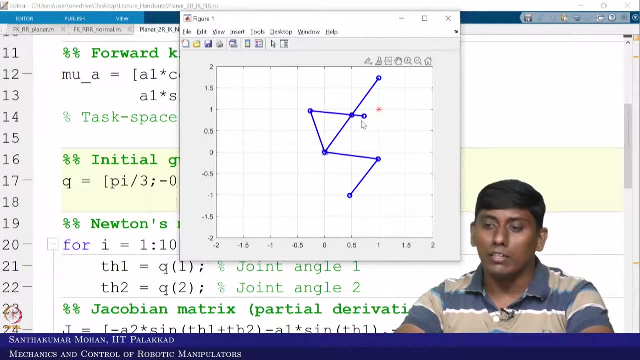 So now, for example, I am taking a different initial guess in the sense I am taking this is actually like a 0, the theta 2 is actually like 0. can I get convergence? I can see. So it is something like that. If I start with 0, so you can see, your Jacobian matrix is actually like going to be non invertible. 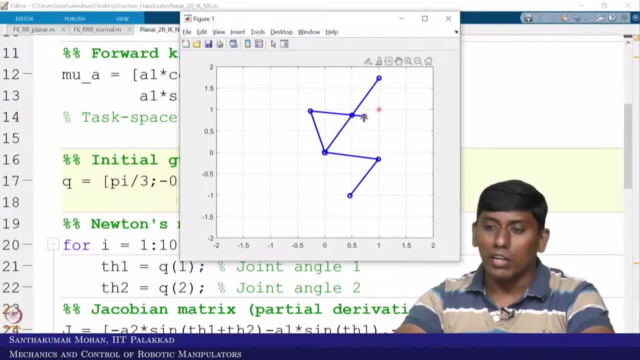 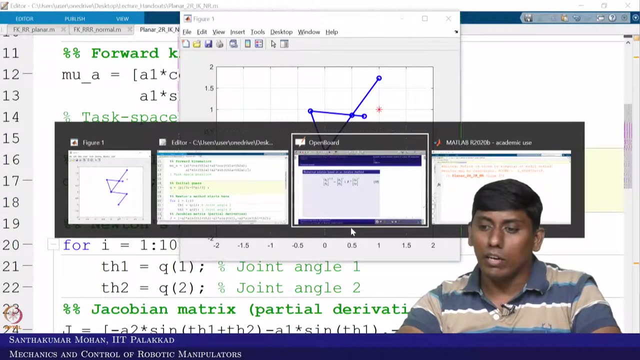 form. It is still, it is actually somehow managed and it is actually like coming. you can see, like keep getting it right. So the third iteration has come, Ok, And the fourth iteration is not reached. we can see. is there any reason? yes, we have actually. 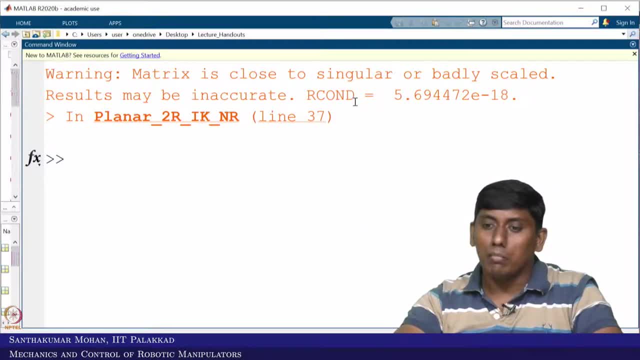 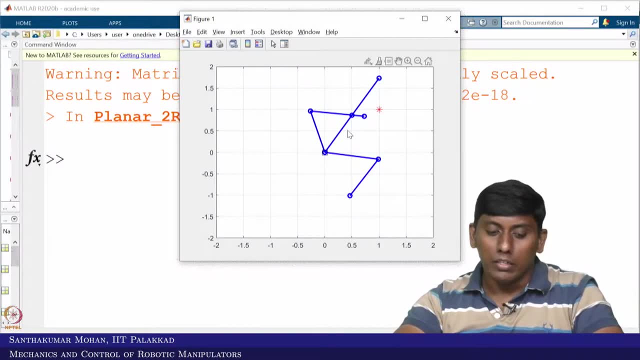 like a reason, right? So it is actually like matrix is much closer because we started with what you call the non, this singular point. So now, in order to make it that much more So, I am actually like assuming that this is something like 0.2. ok. 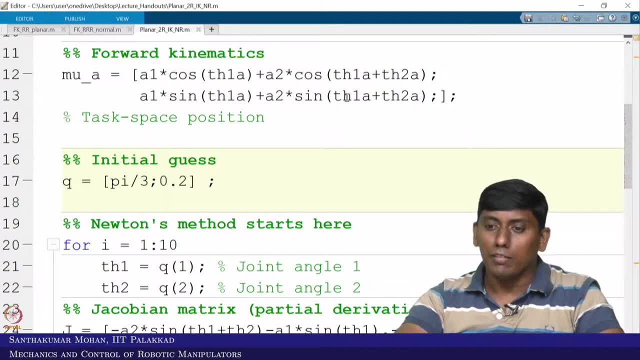 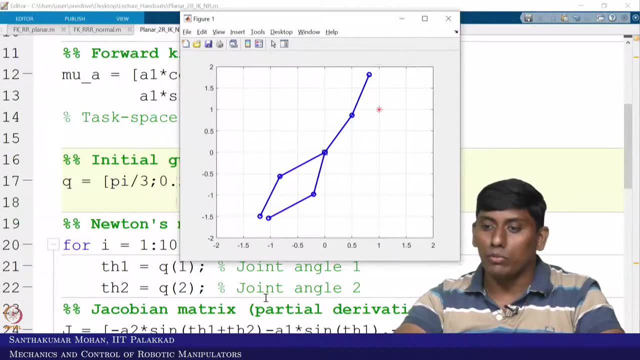 So I am just running it Ok. So you can actually like see this is the first, the second it is going the exact opposite solution. So you can see like it is actually like ending with something like somewhere where the result is actually like inflection kind of thing. 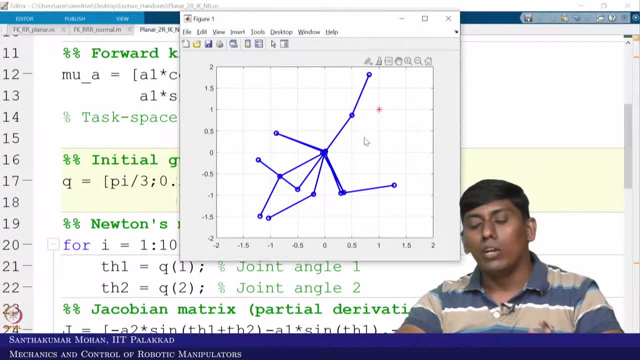 Your initial starting point, or the guess is actually like closer to the inflection point. So that is why you can see even the tin iteration is not sufficient. Ok, So you can actually like see it is keep going, So probably It may end if I increase the iteration count. but you can see, right, it is actually like 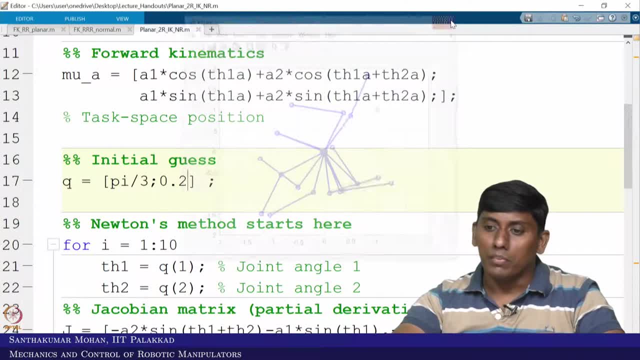 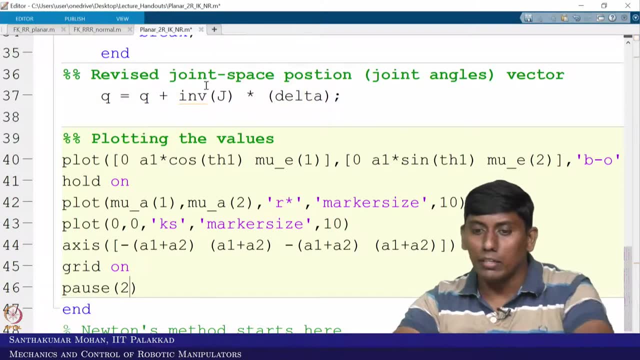 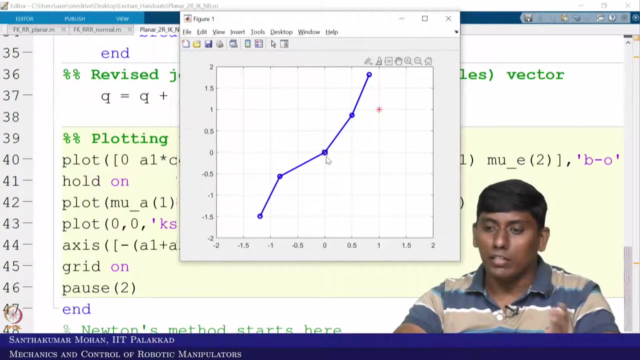 one iteration to another iteration. it is actually keep going. So even I will actually like increase this, ok, and I will actually like make this delay probably 2 second. So I am just running this, ok, So you can see, this is the starting point. this is the next iteration. this is next iteration. 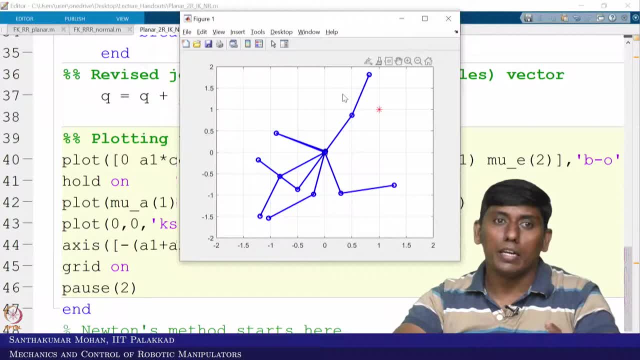 and you can see this is the next And it is actually like keep going Again and again. ok, So you can actually like see. it may actually like converge or not. you can actually like see because we increase the count right. So now it may be, but the initial guess is actually like around the inflection point. 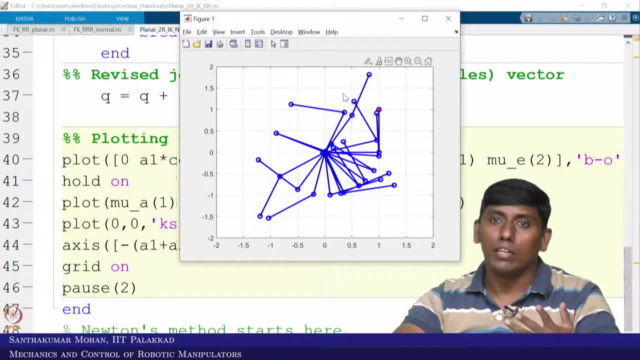 it may actually like take time. you can see, it is actually like converge, right, But it takes more iterations, right. but earlier case you start the initial guess very closer, You got it find immediately with the 3 or 4 count. But in this case it is actually like taking a longer time. 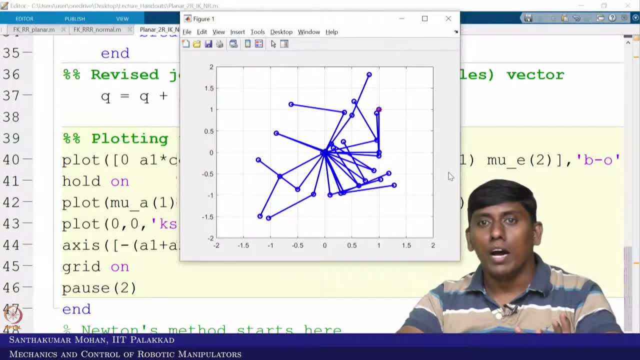 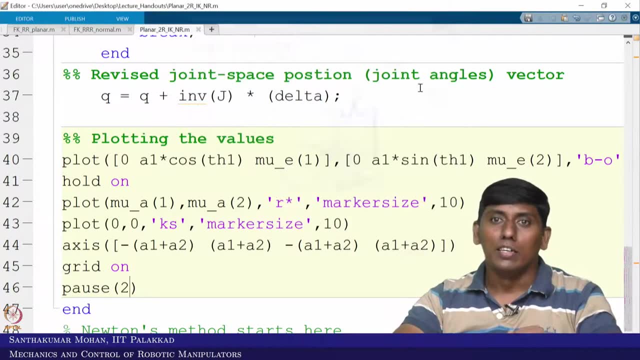 So it is actually like it taken longer duration to do this. I hope now you actually like understand what is this Newton Raphson method is doing it and you can actually like change even this target. So, for example, this is: we have given this way, right. 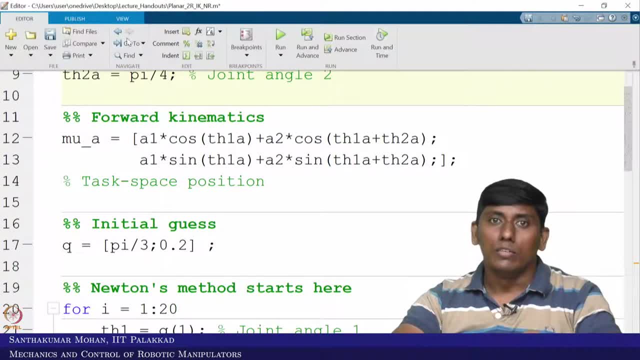 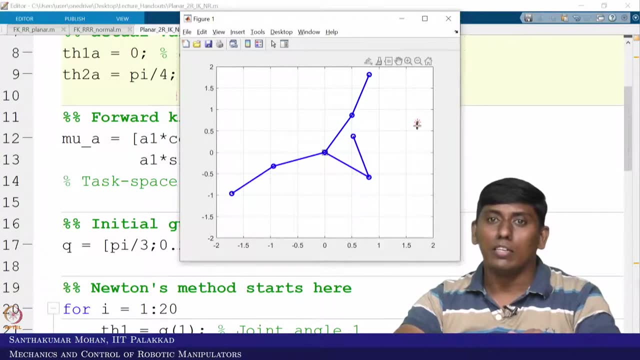 So now I take this as a point. ok, So now in the sense the my, the mu point has changed. So earlier is somewhere here, So now it is changed here. So probably it may be taking the iterative count less because it is actually closer right. 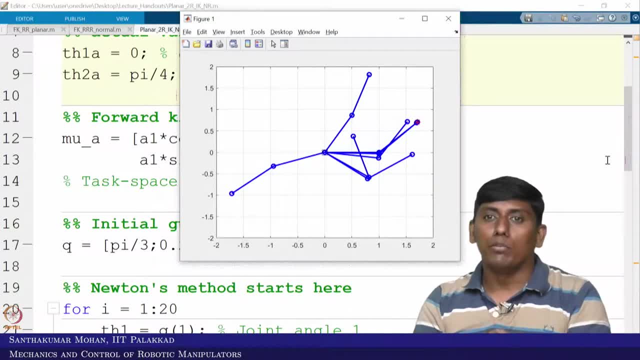 So you can see it takes very less. So that is what. so where your mu and where you are starting. So this will actually like increase the fastness, But still you can see the solution is obtained right in this case. So that is what we are actually like looking at here. 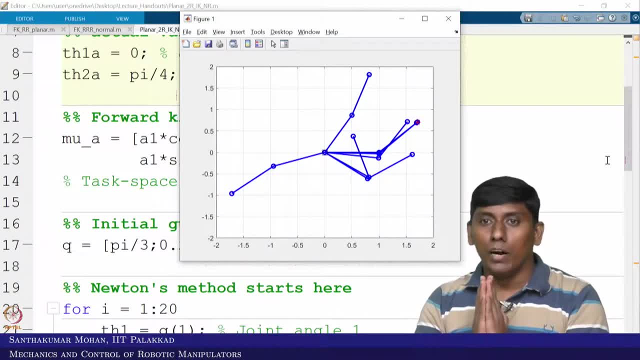 So now I hope you understood what is forward kinematics, What is inverse kinematics, how you can actually like find the forward kinematics using one of the efficient tool called MATLAB. The same way you can see the Newton Raphson method also can be, you can say, embedded in. 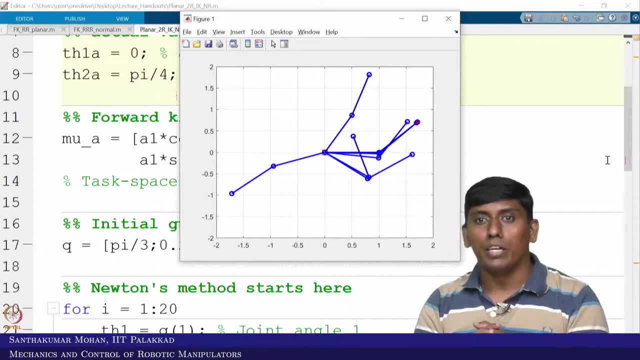 a MATLAB and then you can see the solution is actually like very forward. in the sense it is very easy. I took the example 2R, serial manipulator, because visualization is easy But it is not restricted to only planar or you can say less number of degrees of freedom. 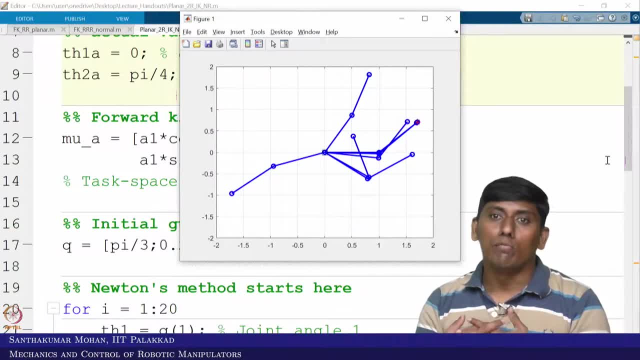 The Newton Raphson method. The Newton Raphson method can be used for any such you can say serial manipulator, okay, So in that sense I hope you are actually like little bit clear. So now even you can see something like close to inflection point. I will give and see that. 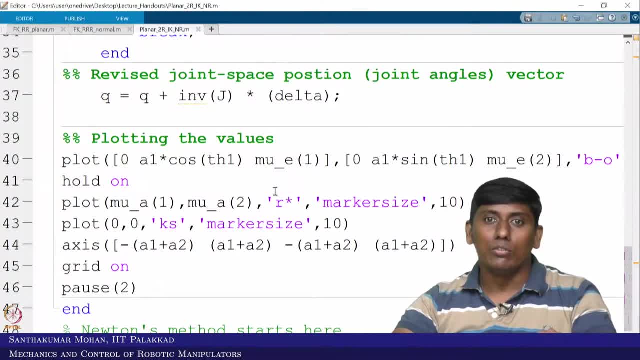 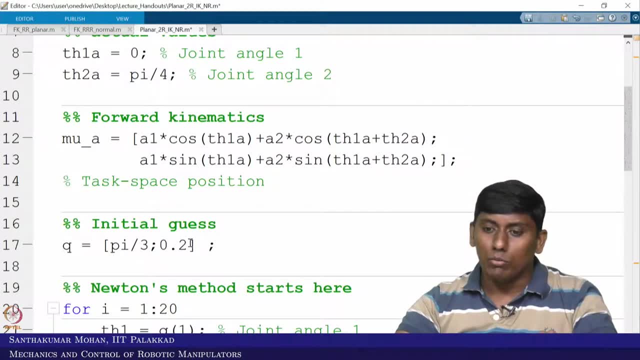 it is actually like keep going. I just to show that. so I will reduce the time, So I reduce the time to 0.1.. So I actually like choose some kind of values, Right? I assume this is actually like non trivial bit, because I do not know, So you can see. 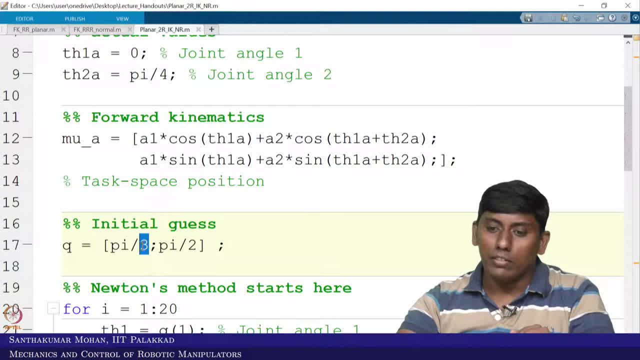 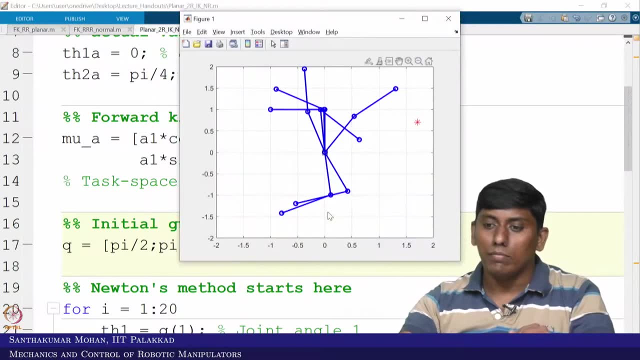 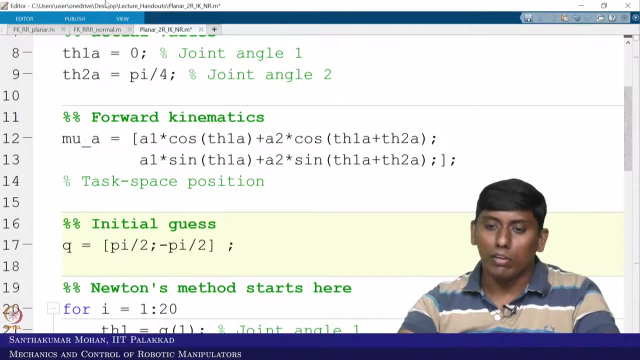 like it is reached right, it is faster. So now I will see this is also pi by 2, ok, So now I am actually giving. you can see right, it is actually like getting the solutions. So now I will see if any inflection point I can actually like end up. ok, It is actually. 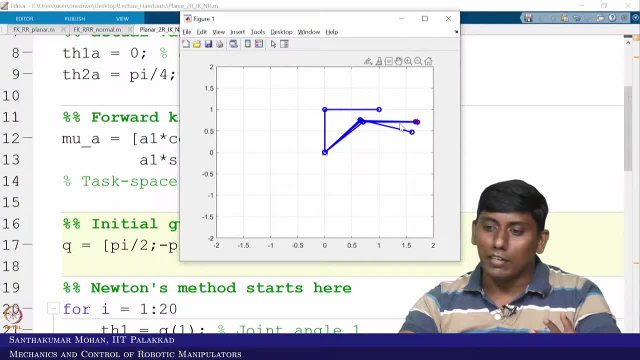 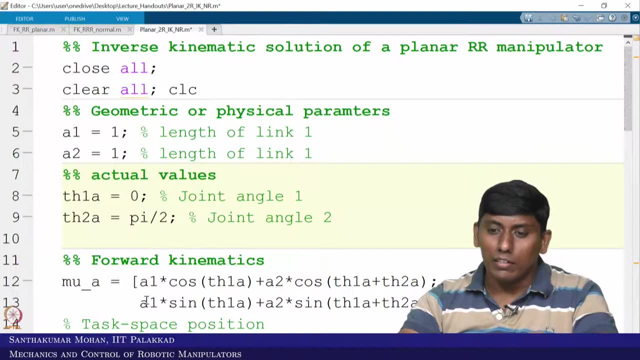 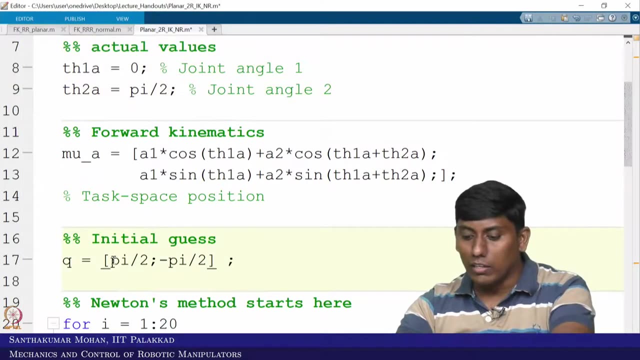 like much faster, right, because you have given the initial guess here and it is you have to move here, right. So now this, I took it, this, So I start. the point is actually like a different, ok, this solution. So I just start this. 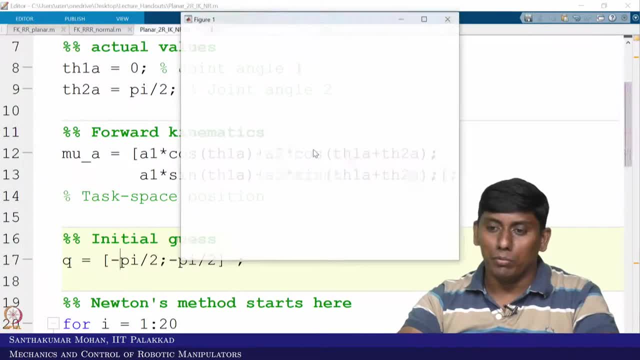 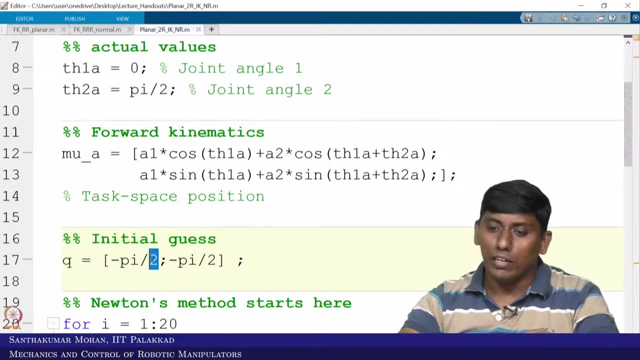 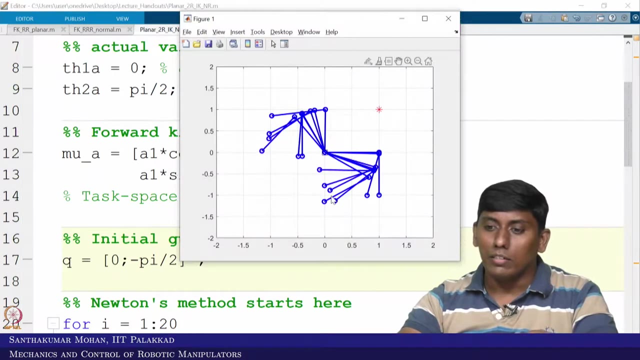 So both are actually like minus pi by 2.. So in the sense I start from here, it is reached right. So now I will start with 0. I am trying to find. is there any inflection which happened to this? yeah, this is the inflection You can see. right, even the 20 iteration is not sufficient. 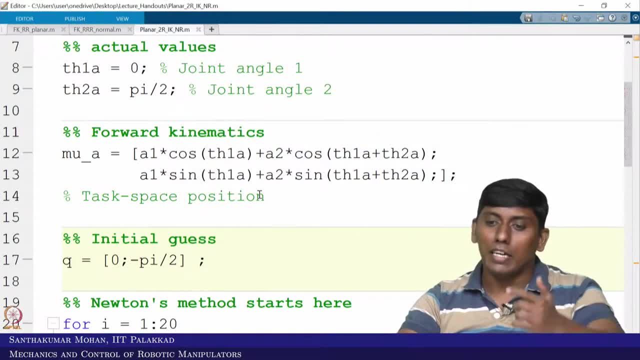 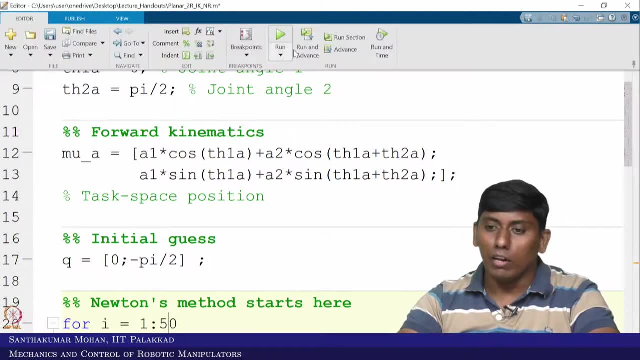 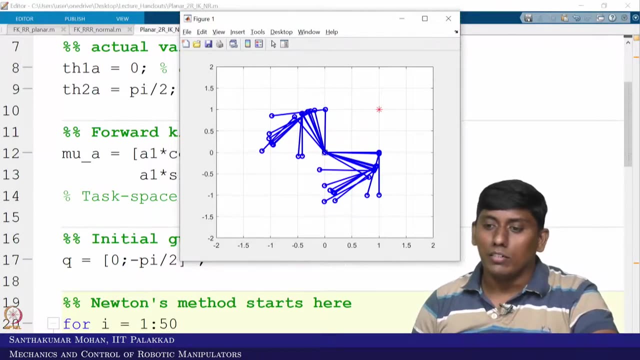 where we have started the initial guess, exactly opposite solution of this. So in the sense, even if I increase to 50.. So if I increase to 50, I do not think it will actually like: come, we will see, right, you can see like it is converge to something that. So it is actually like keep getting. 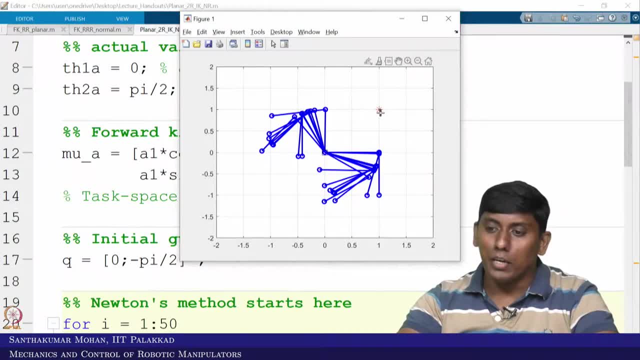 one another solution opposite, because this is the given point but you have taken exactly opposite solution of that. So it is actually like it is actually like never end. this is another solution which is actually like come under as a inflection. So because of that, 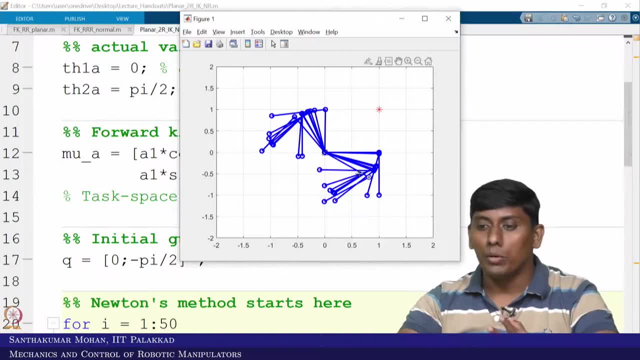 you can see it is keep coming and it is ending with the same thing. ok, So this is the way. So this is the way we can actually like. see, the Newton Raphson method is very much beneficial for us and you can see that the code, what we have written, is actually like very straight. 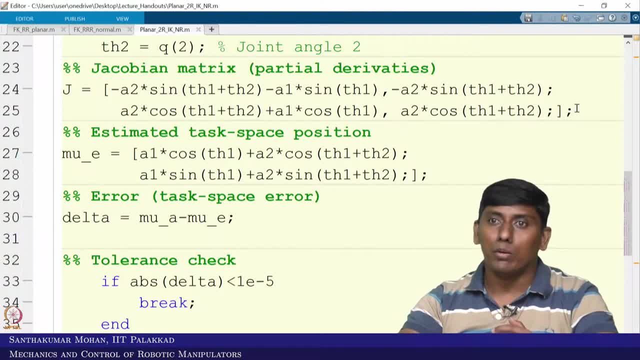 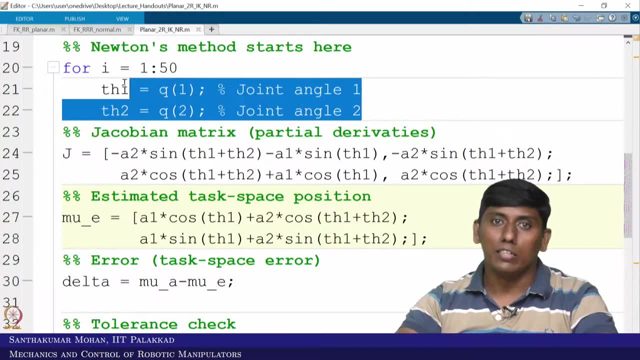 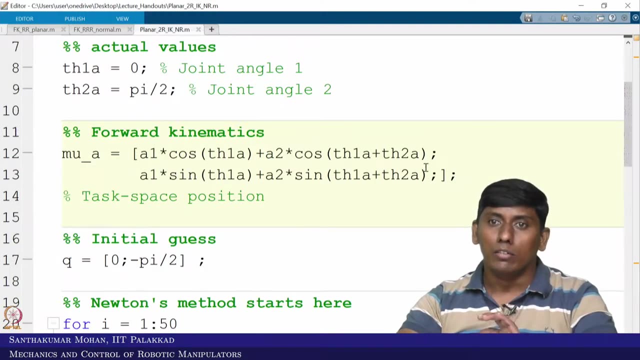 forward. So if you want to use any other manipulator, this Jacobian will get changed and this mu vector will get changed, and this would be changed. The remaining everything is same. in fact, this mu actual would be given to you as a direct value.